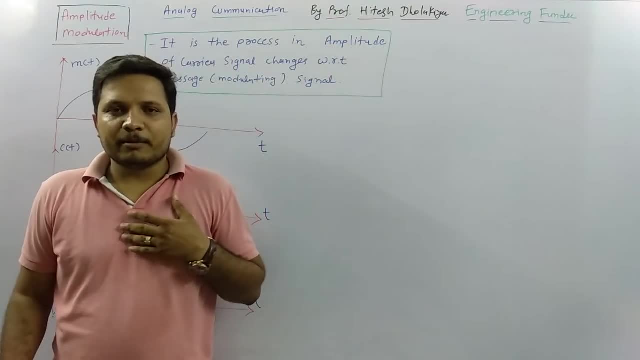 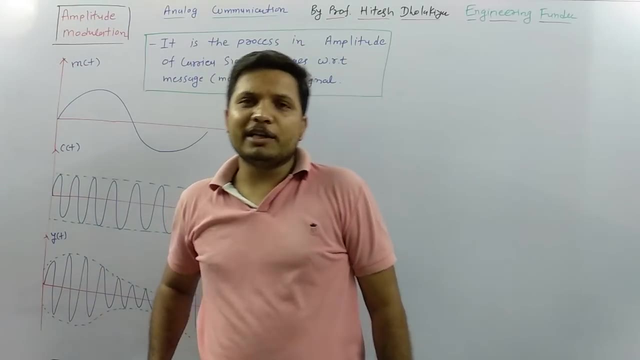 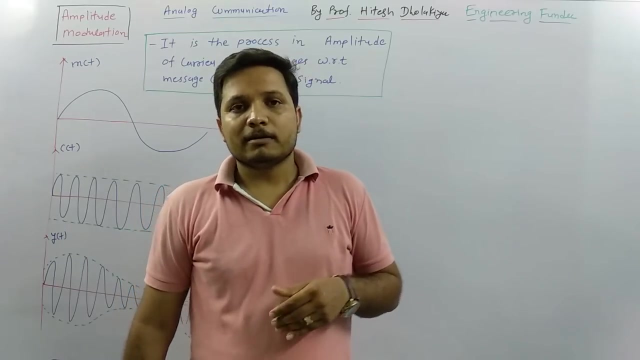 Welcome to Communication Engineering playlist. Here in this session I'll be going to explain amplitude modulation. So in this session first I'll explain what is the basics of amplitude modulation, Then after I'll explain how physically signal is getting changed in amplitude modulation. 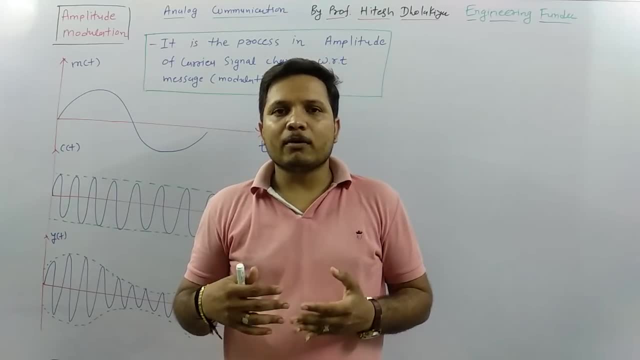 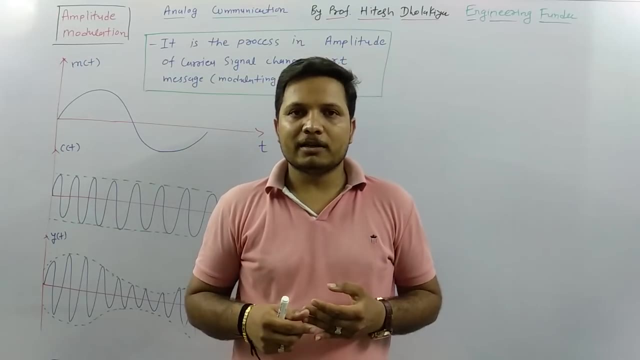 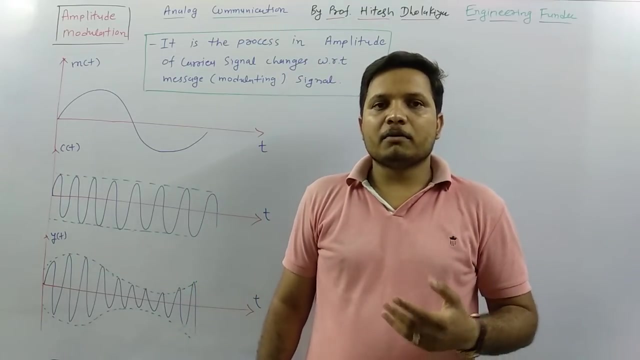 Then after, we will derive basic equations, which is very helpful to solve out problems based on amplitude modulation, And then at the end, I'll sum up this session by frequency response, which is there with amplitude modulated signal. So let us begin this session with basics of amplitude modulation. 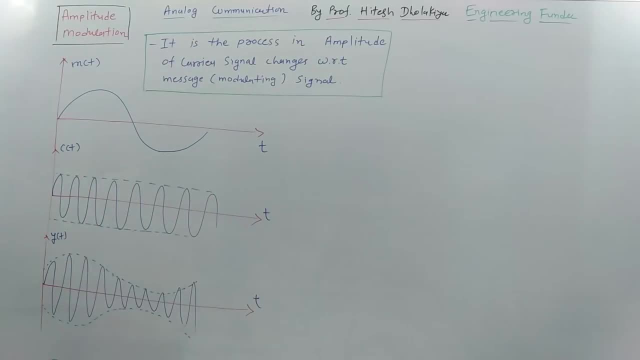 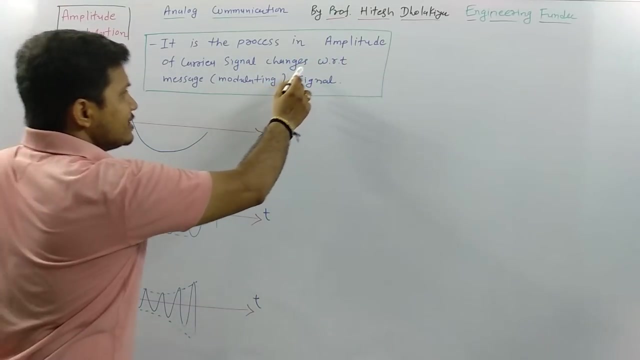 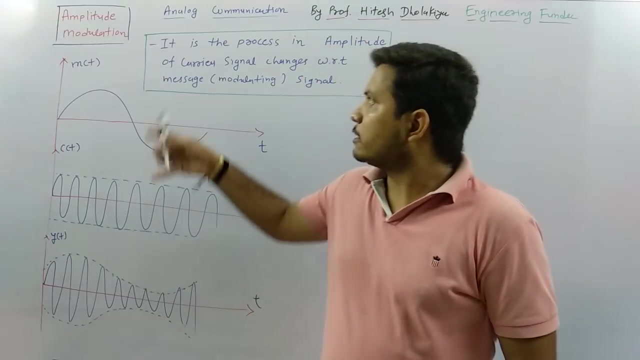 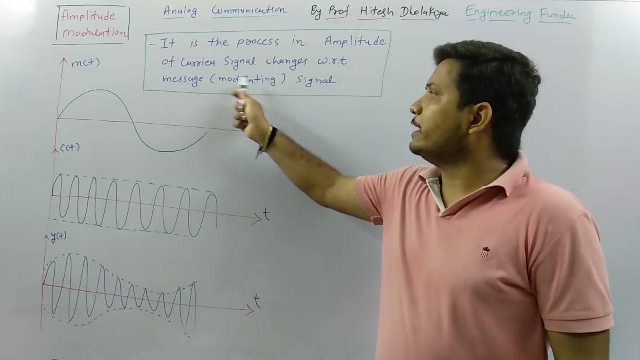 So, first of all, what is amplitude modulation? So amplitude modulation is a process in which amplitude of carrier signal changes with respect to modulating signal. So here in amplitude modulation, amplitude of carrier signal get modifies with respect to modulating or message signal. 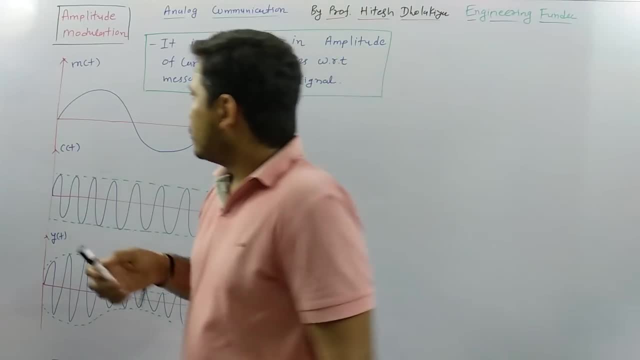 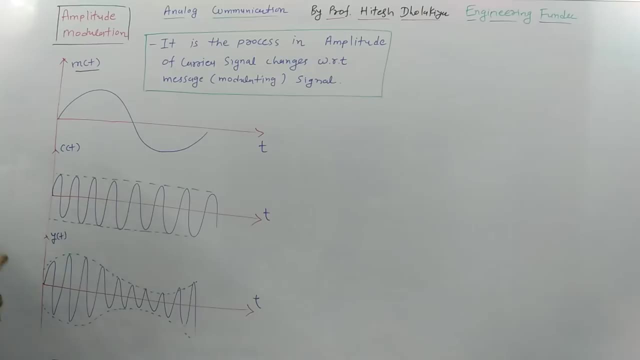 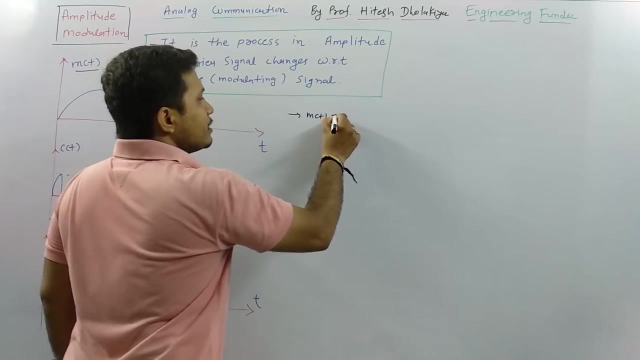 So this is what the basic process which happens Now here, as you can see, this is what modulating signal is. So this is modulating signal. MT. So this is modulating signal. MT. So MT, that is modulating signal. 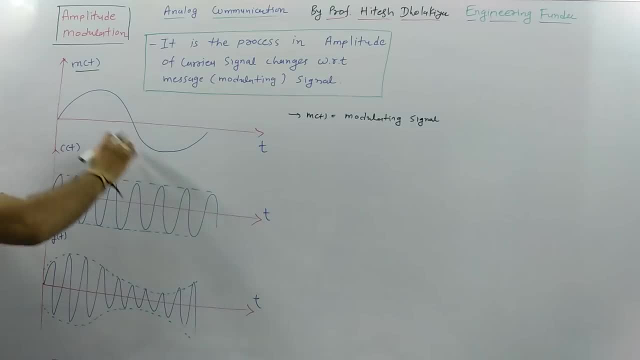 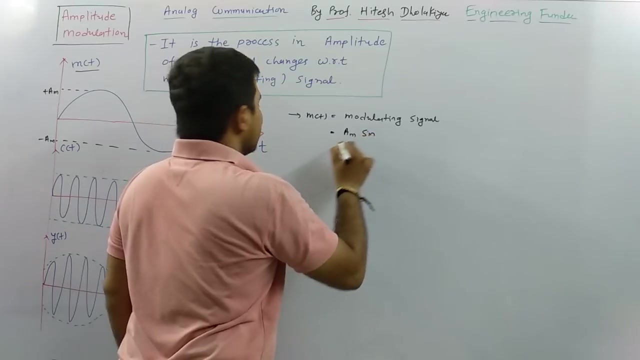 Now, as one can see, this modulating signal is low frequency signal And if I say it's amplitude, that is varying in between plus AM to minus AM, and that is what sign signal. So that signal is AM sine. if I say its frequency is omega M, 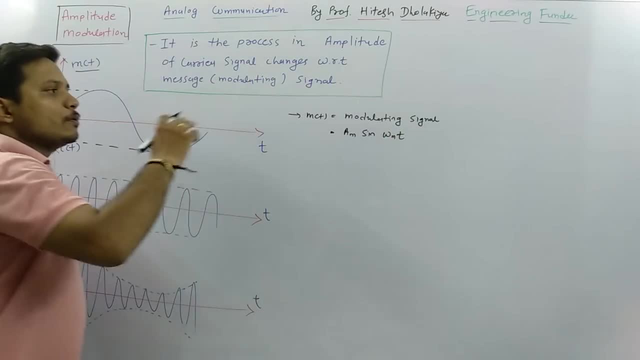 then omega MT, So modulating signal, that is AM sine omega MT. This is carrier signal, that is high frequency signal. So this carrier signal, that is high frequency signal- one can clearly see number of cycles- are quite more than modulating signal. 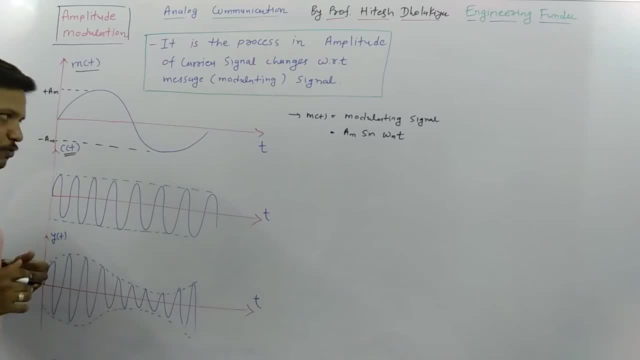 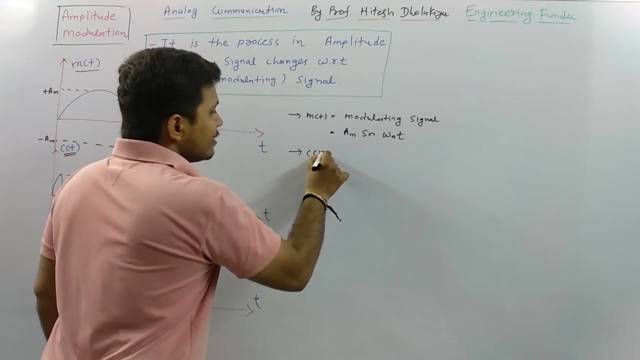 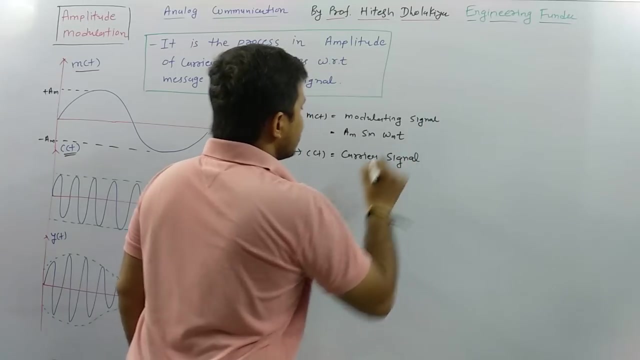 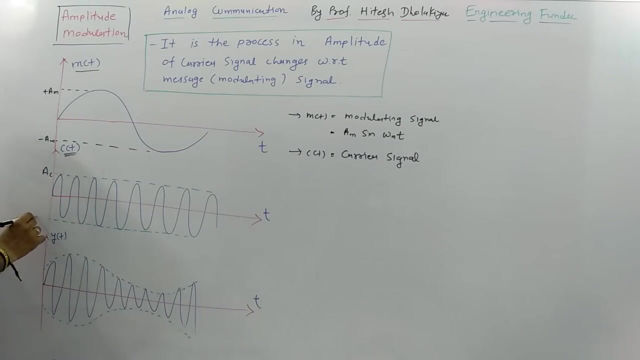 And that is what the basic agenda which is there with modulation process. So here this CT, that is carrier signal. So CT, that is carrier signal, And if I say its amplitude varies from plus AC to minus AC, And if its frequency is omega C, 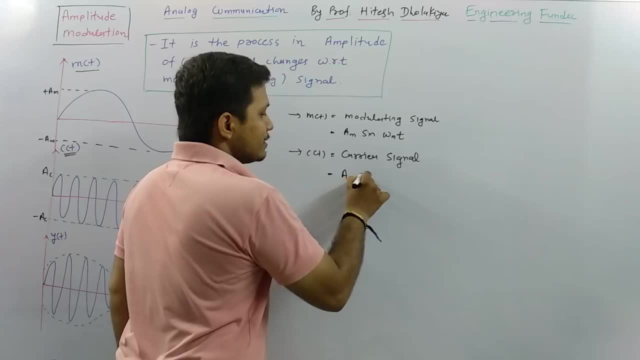 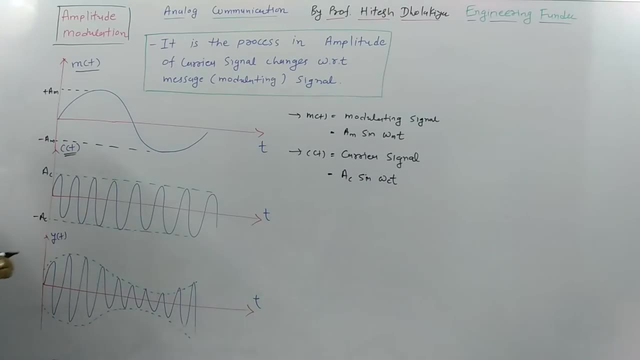 then we can say it is AC sine omega CT. Now here this YT. is what Amplified modulated signal? Now here one can see this YT. that is what having frequency similar to carrier signal. So frequency of carrier signal and modulated signal, both are same. 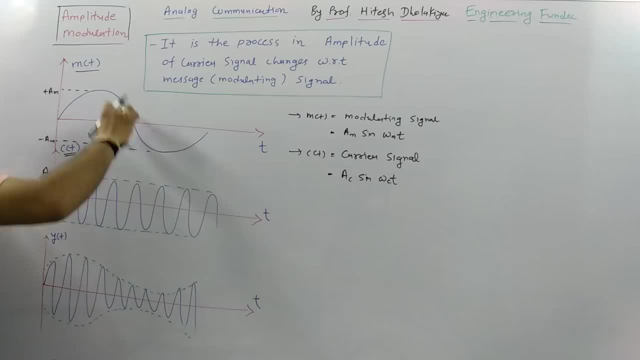 But amplitude of carrier signal. that is changing with respect to modulating signal. So one can see here, this is how amplitude is changing, Where here modulating signals amplitude is changing like this, And carrier signals envelope. this is what we can say, envelope of carrier signal. 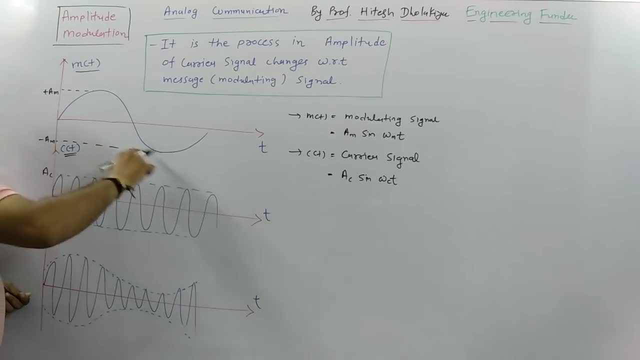 So that envelope of carrier signal that is changing as amplitude of modulating signal. So amplitude of carrier signal changes as per modulating signal, And that is what amplitude modulation process. Now here, one basic thing that we need to focus about: 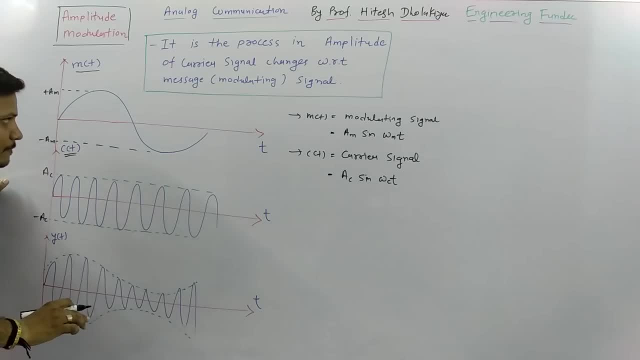 Like: see this amplitude of carrier signal is AC And that is varying from plus or minus AC. like this And modulating signal that is having amplitude which is varying from plus AM to minus AM. So here, at this instant, amplitude of this modulated signal, that is maximum. 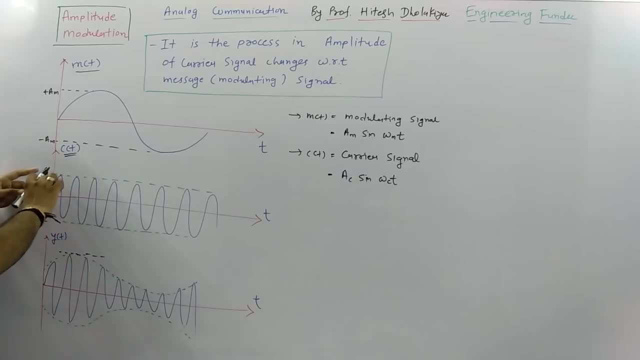 So what has to be this amplitude? That should be AC plus AM. So this amplitude of this modulated signal, that is AC plus AM, While over here one can see amplitude of modulating signal is minimum, that is minus AM. So over here envelope of carrier signal that will be having amplitude that is AC minus AM. 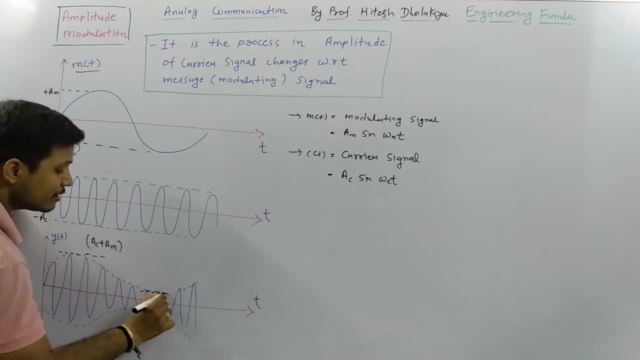 So this amplitude that will be AC minus AM. So this is what amplitude of amplitude modulated signal over here. So ultimately you will be finding amplitude of carrier signal, Means envelope of amplitude that is getting changed with respect to modulating signal. 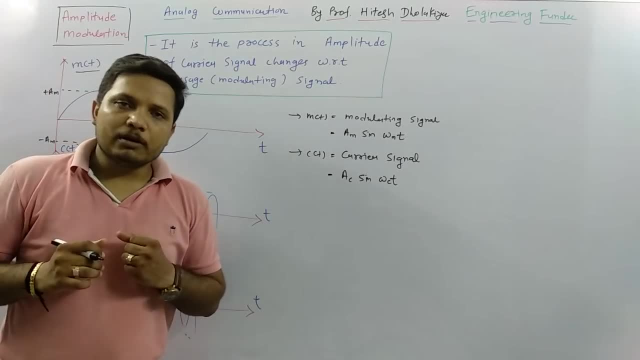 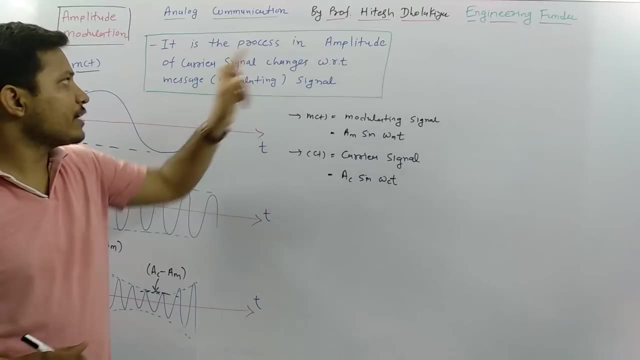 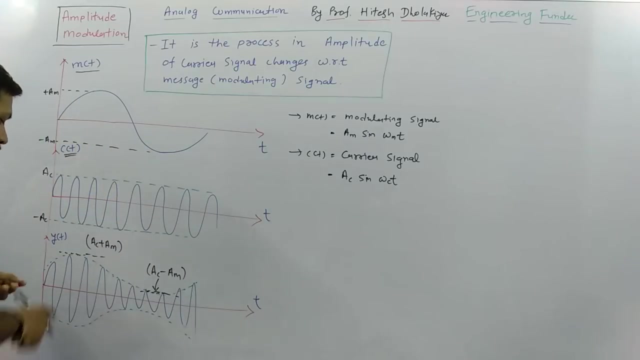 And that is what the basic process which is there with amplitude modulation. So amplitude modulation, that is a process in which amplitude of carrier signal changes with respect to message signal. Here message signal is empty And amplitude of carrier signal that is getting changed. 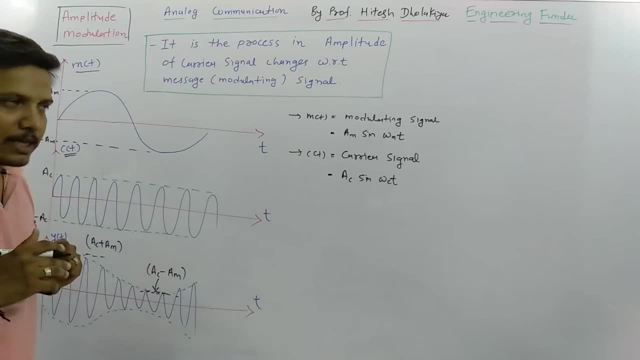 With respect to message signal. that is what the basic process which is happening here. Now I will be deriving this equation of amplitude modulated signal. So what will be amplitude modulated signal? So that is what I will be explaining here. 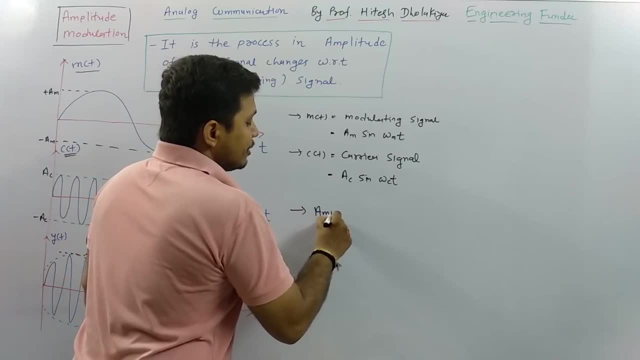 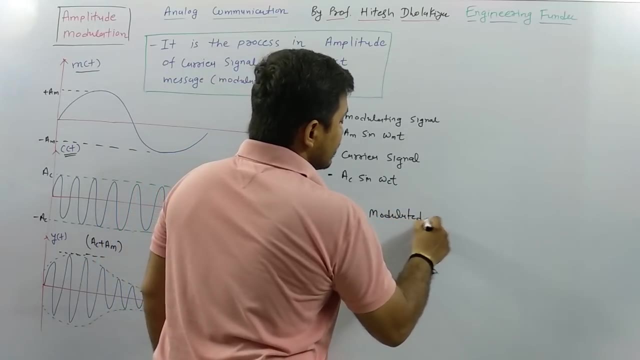 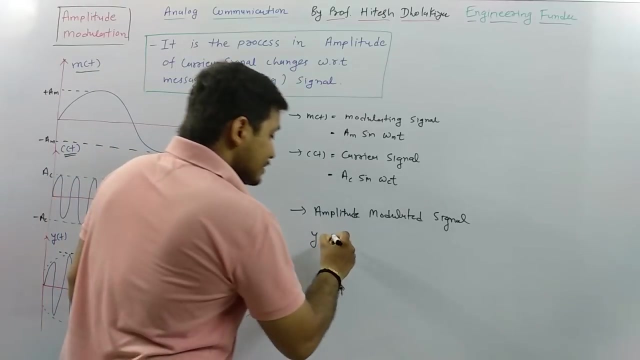 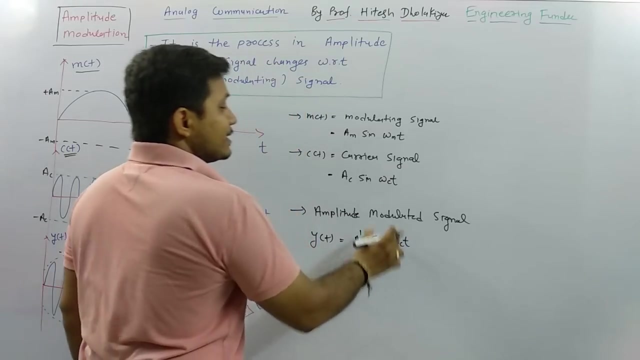 So amplitude modulated signal, So that will be. if I say that is YT, So that is. let us say it is A dash, Its frequency is not changing. So omega CT, So carrier signal's frequency, that is not changing. 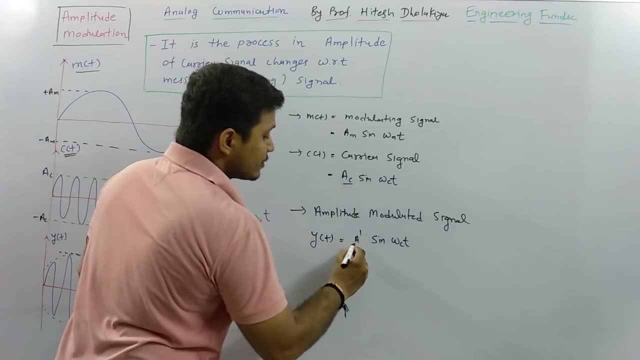 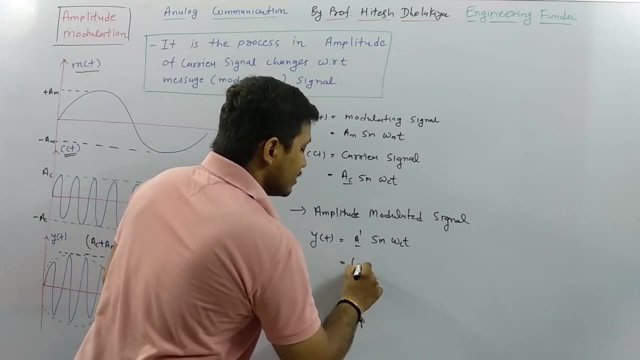 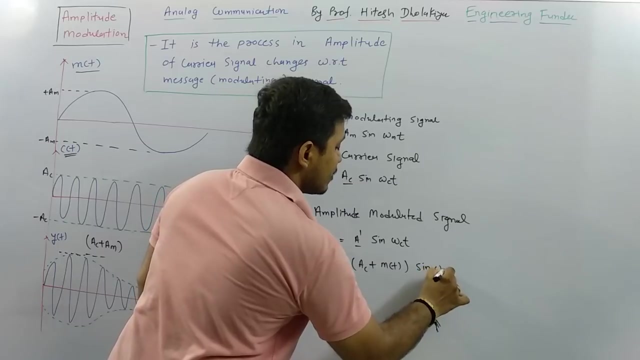 What is getting change of carrier signal Amplitude. So now new amplitude is A dash. Now how it is getting change. So that is getting change as per AC plus modulating signal's amplitude, MT. So this is what A dash. 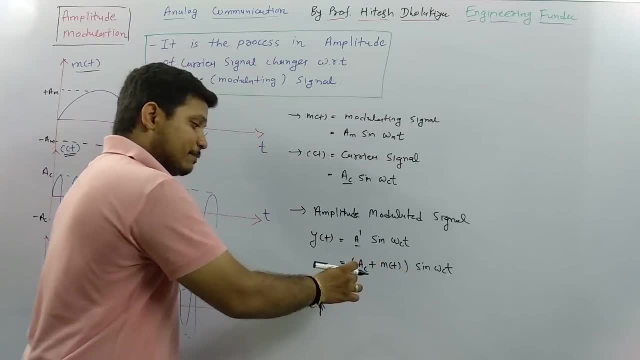 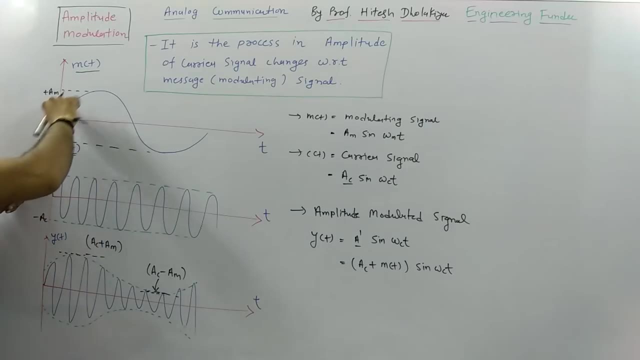 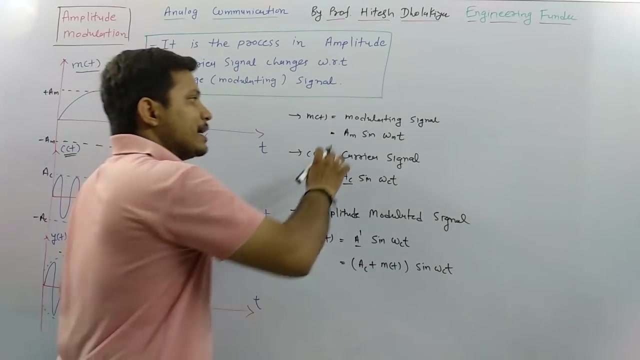 So that A dash that is changing as per modulating signal MT, So that A dash is AC plus MT. So this is what amplitude modulated signal Now, as I have to modulating signal that is AM sine omega, MT. 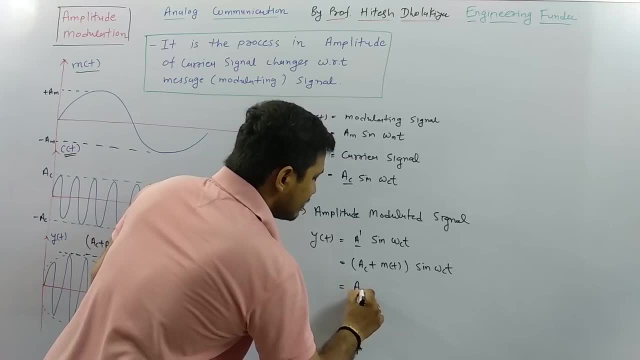 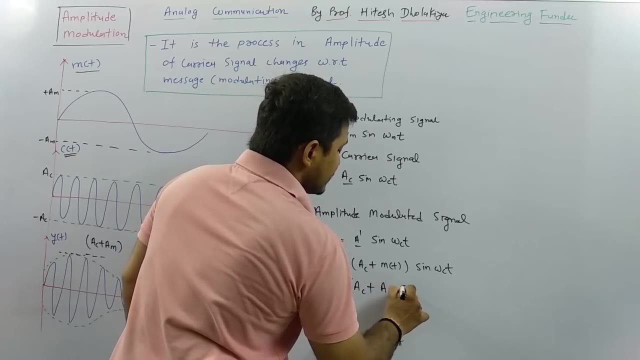 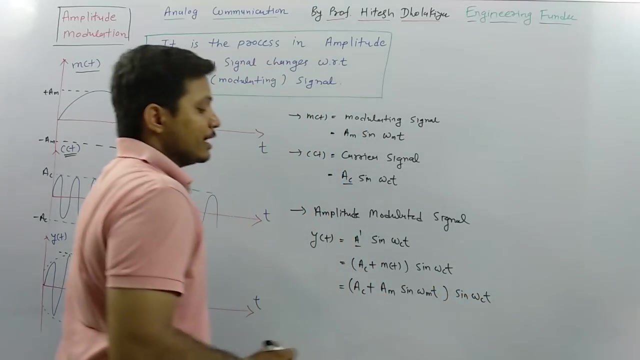 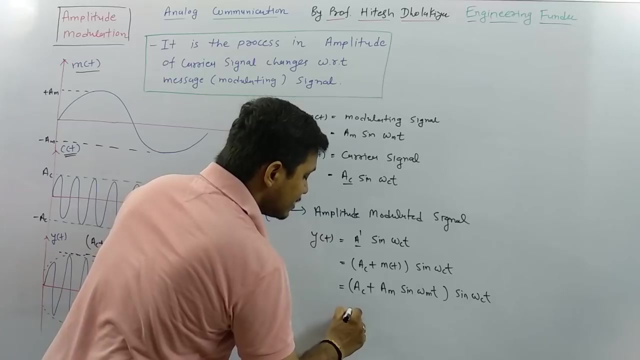 So just place this in this equation. So it will be now AC Plus MT is AM sine omega, MT into sine omega CT. Now here, if I take AC common from this counts. in that case Now it will be AC common. 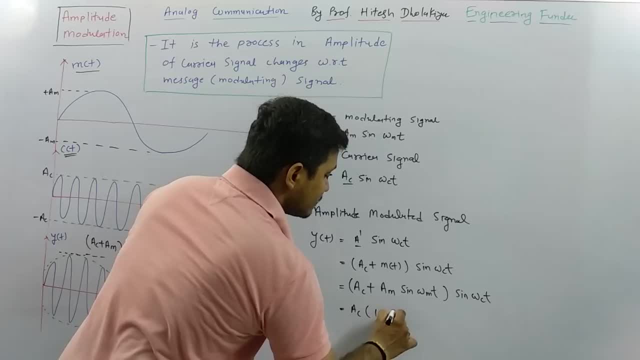 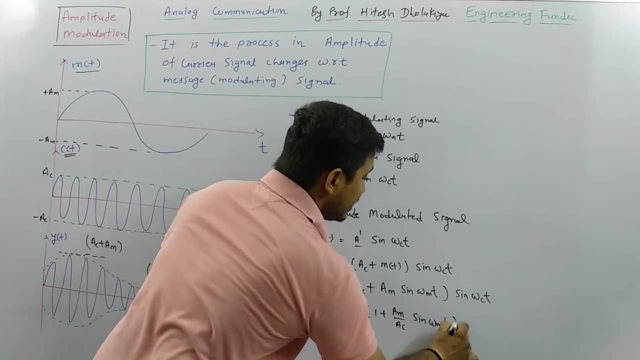 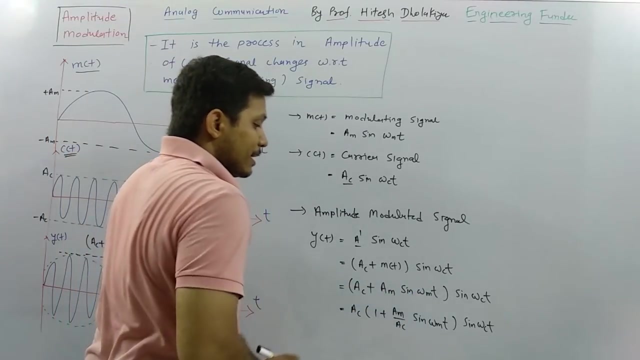 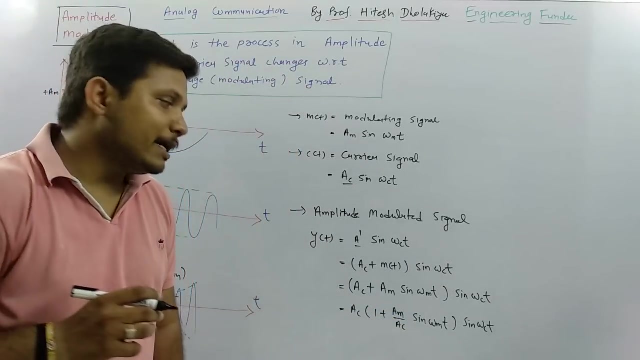 Take it outside Now this will be 1 plus AM divided by AC into sine omega MT, Into sine omega MT into sine omega CT. So this is what my amplitude modulated signal Now here: AM by AC, that is modulating index. 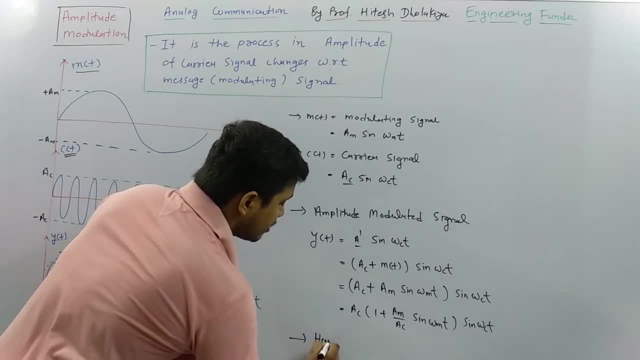 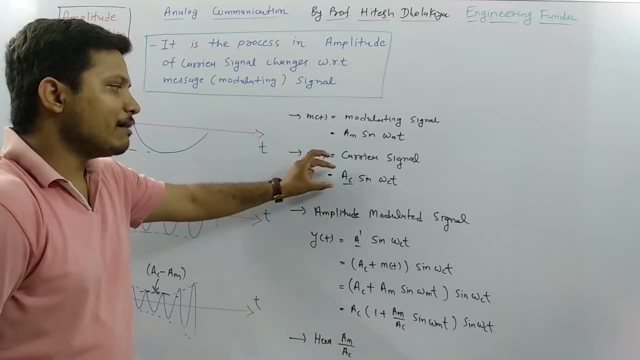 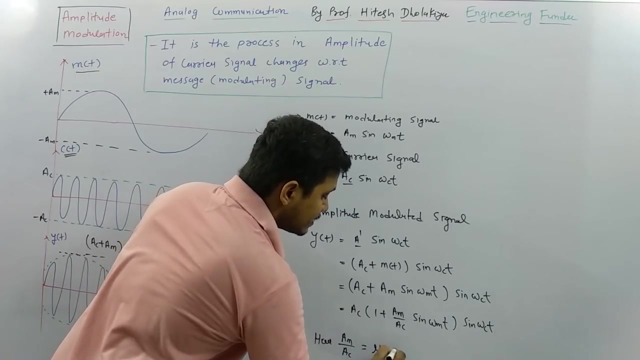 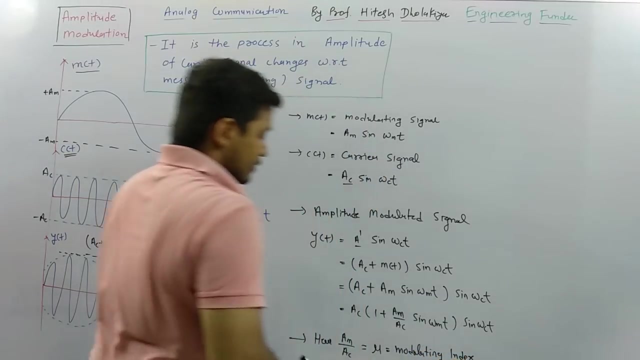 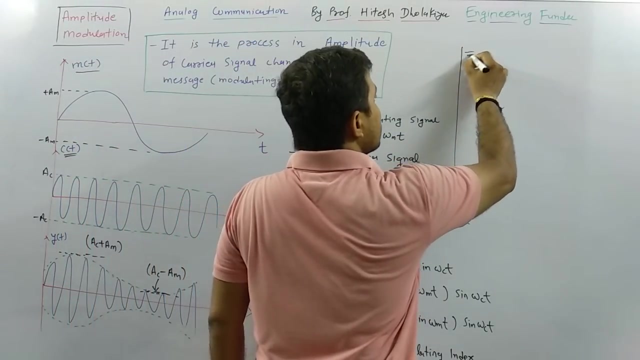 Here, AM divided by AC Means amplitude of modulating signal divided by amplitude of carrier signal. that is modulating index. So let us say this is mu and that is modulating index. So now this equation of modulated signal, now that will changes to. 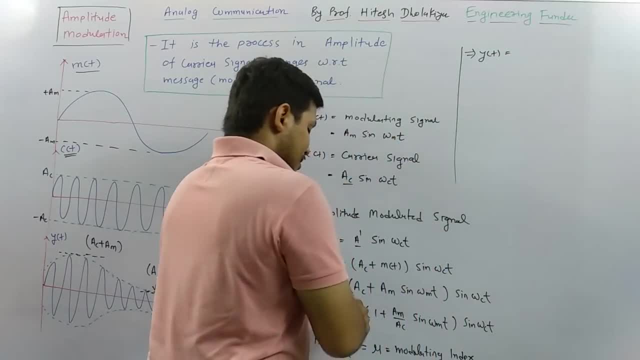 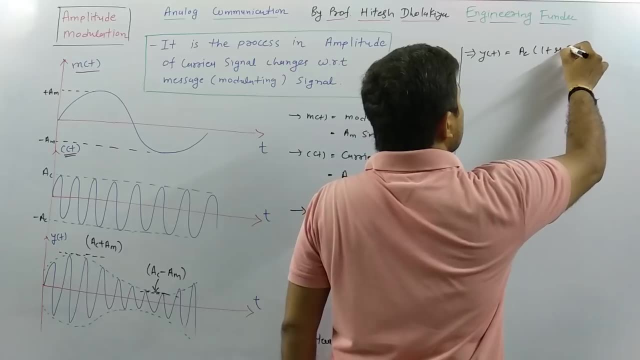 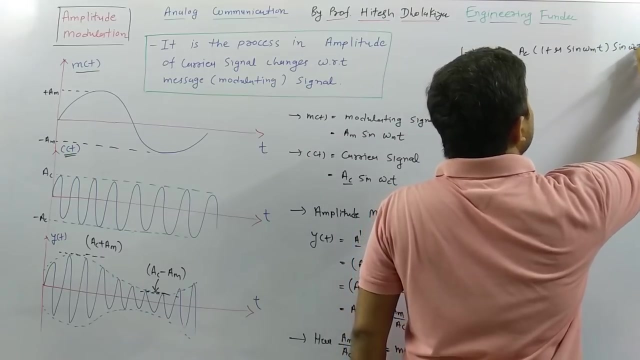 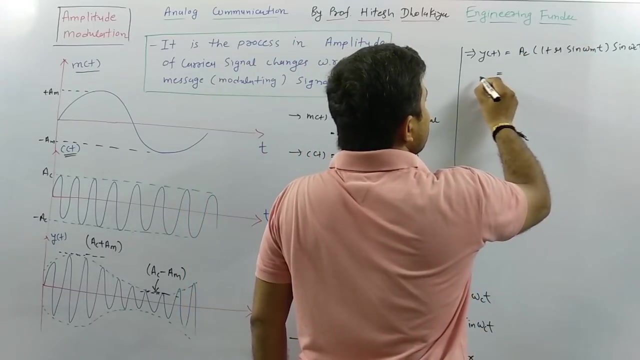 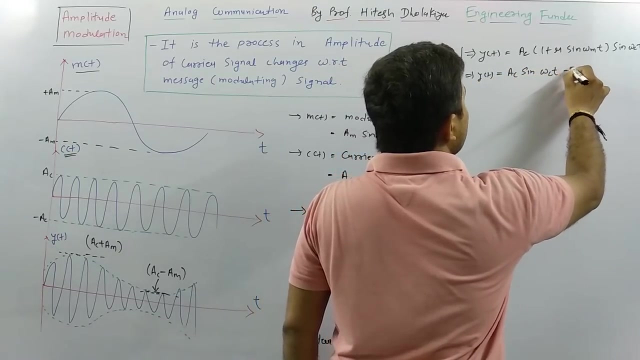 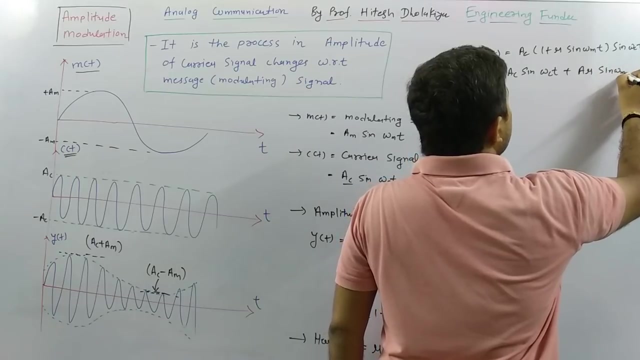 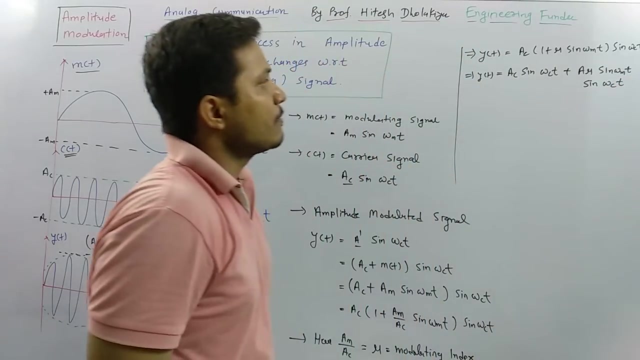 Yt is equals to AC into 1 plus mu sine omega MT, into sine omega CT. Now here just resimplify this. So Yt, that is AC sine Omega CT plus A into mu, into sine omega MT, into sine omega CT. 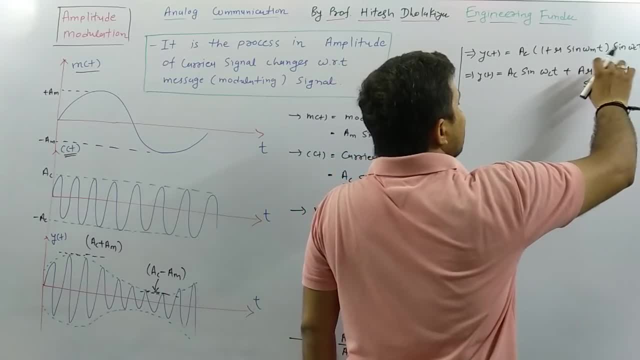 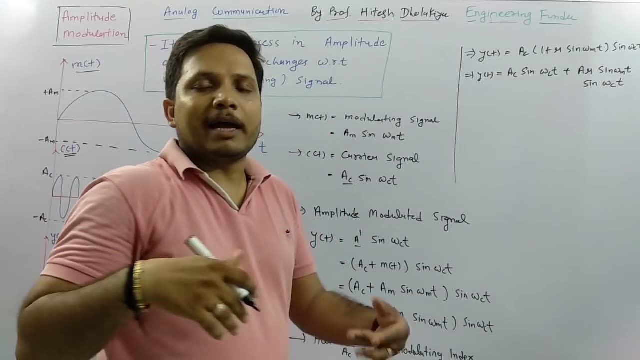 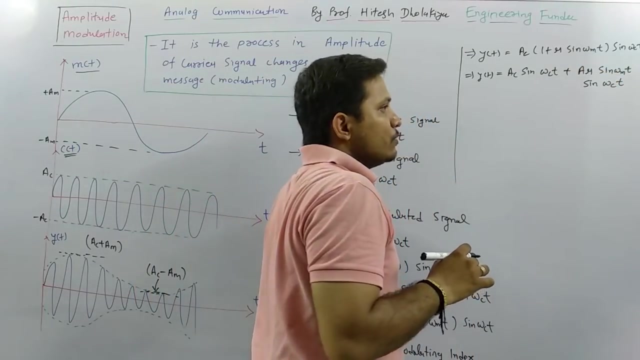 Now what I will be doing here. I will be taking this signal in terms of frequency components And to have that signal in terms of frequency component, I will be doing this: 2SS is equals to C minus C- Sorry- minus C plus C. 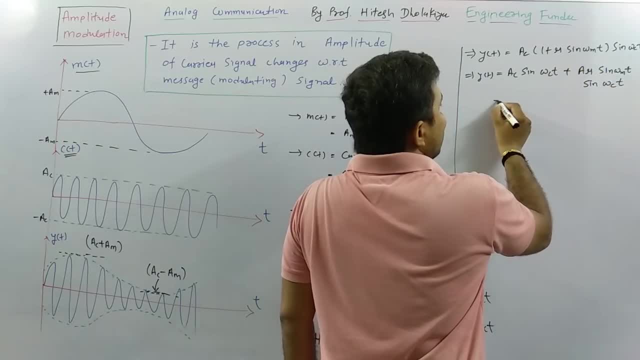 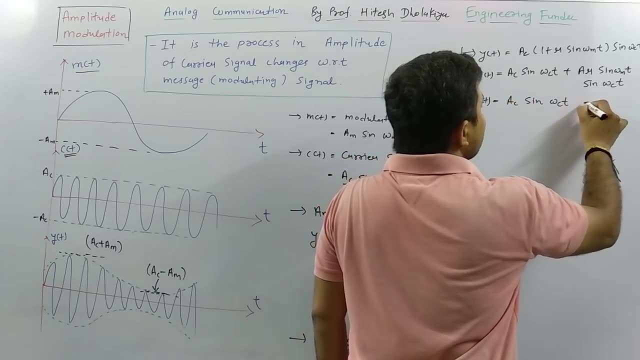 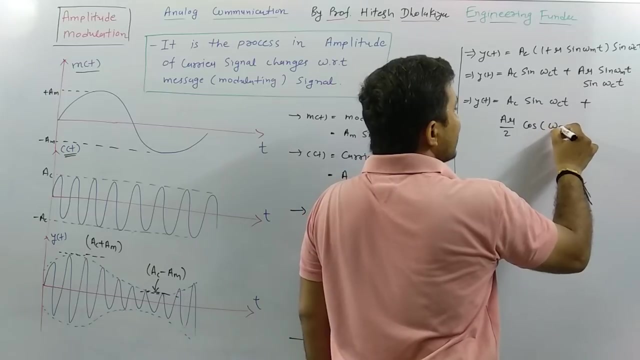 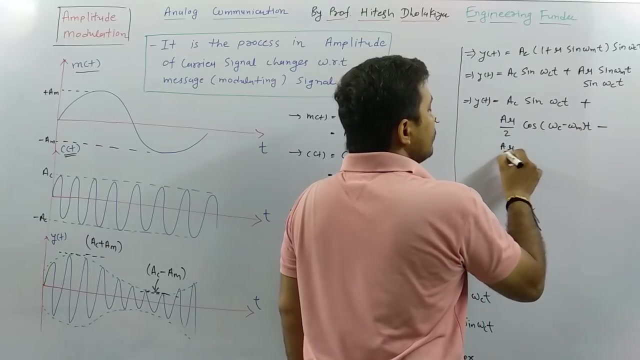 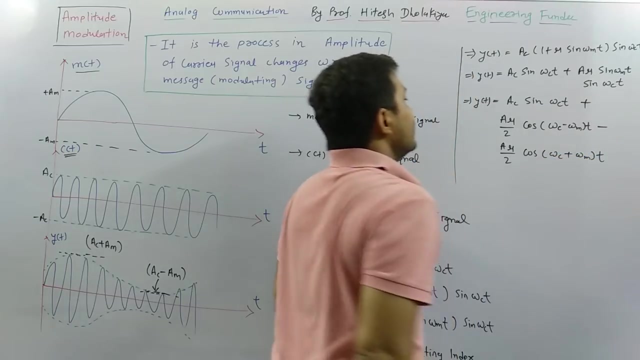 So just multiply 2 and divide 2.. So that will result into Yt. That is, AC sine omega CT plus A mu by 2.. Into cos omega C minus omega MT Minus A into mu by 2.. Into cos of omega C plus omega MT. 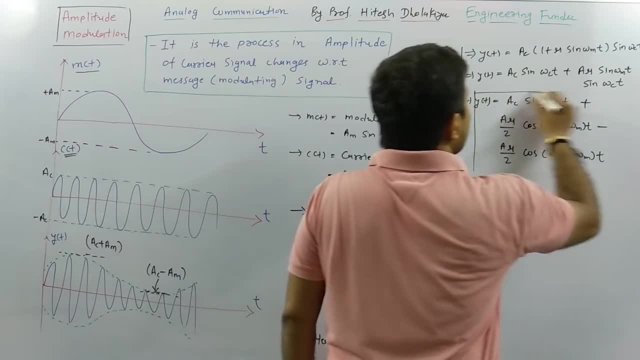 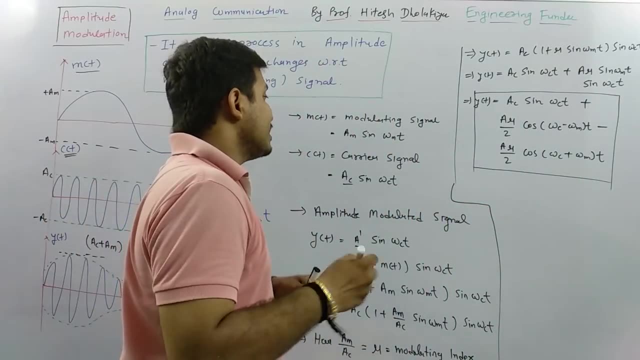 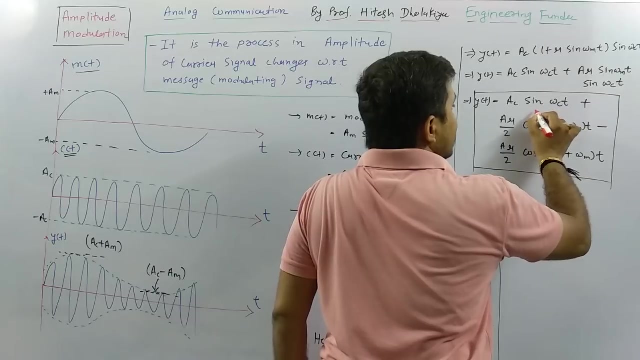 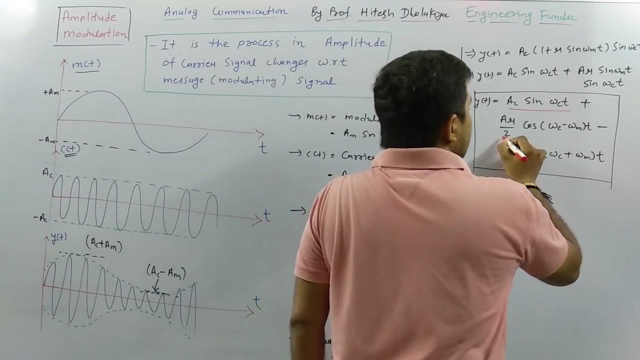 So this is what my basic equation of amplitude modulated signal. Now here one thing that is clearly visible, That is this signal that is having 3 different frequency components. One is AC sine omega CT. Second is mu A by 2 into cos omega C minus omega MT. 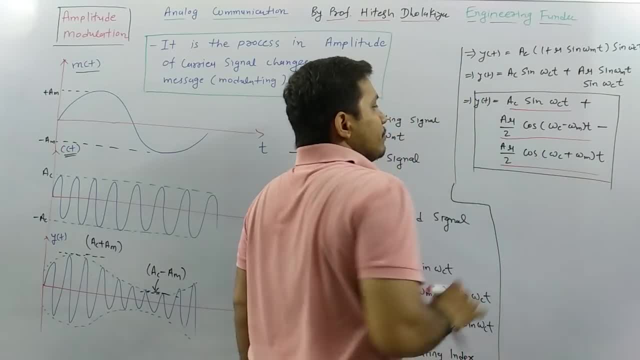 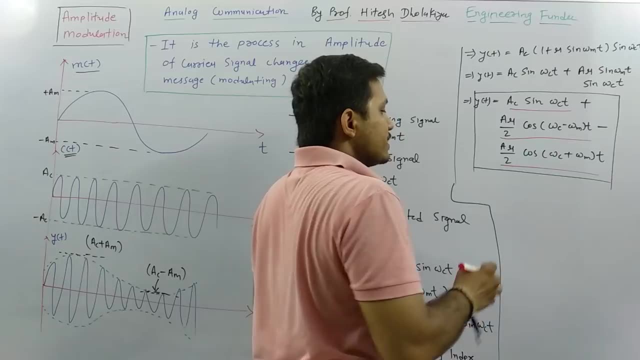 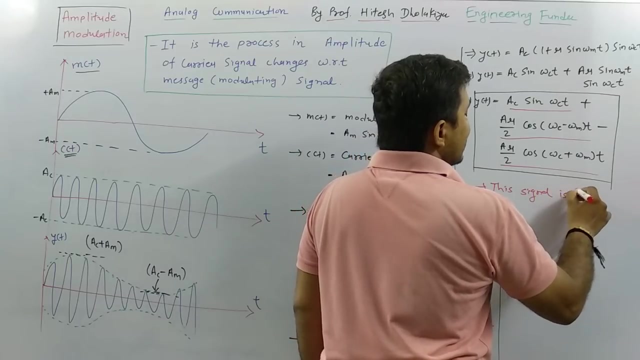 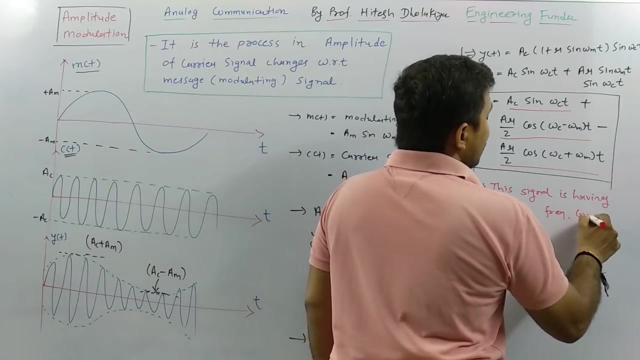 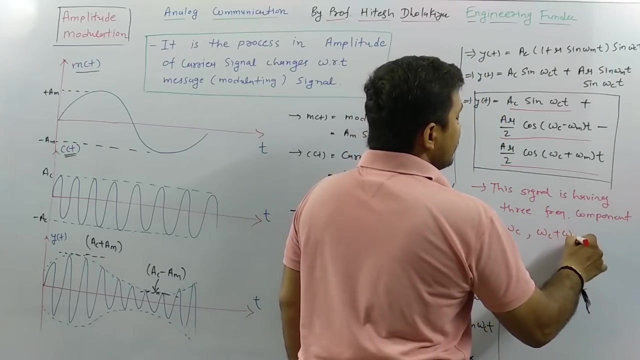 And this is mu A by 2 into cos of omega C plus omega MT. So this signal is having 3 frequency components. This signal is having 3 frequency components And that is omega C, omega C plus omega MT and omega C minus omega MT. 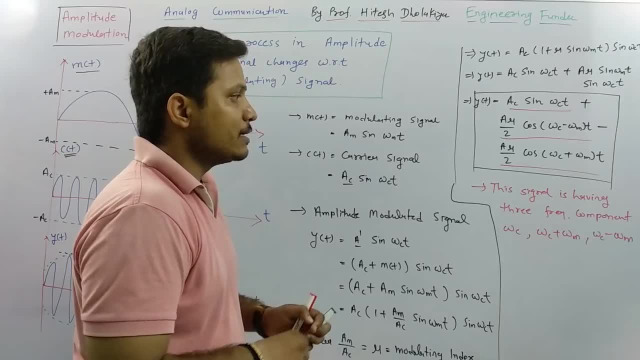 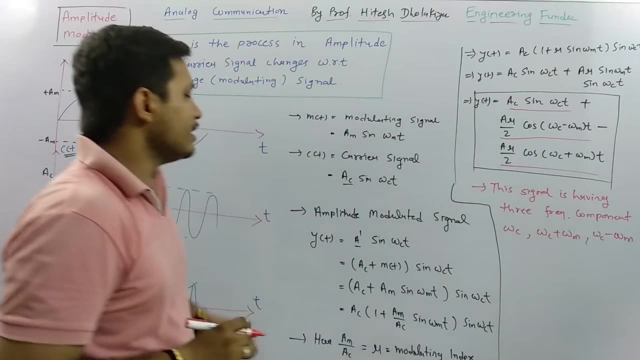 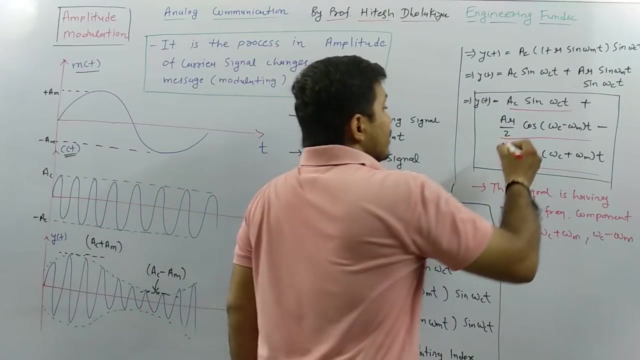 So this 3 frequency components are there with this signal: This omega C, that is what carrier signal, which is even we are transmitting in AM signal, And that is having amplitude AC, which is what amplitude of carrier signal, And this frequency component, which is what sidebands. 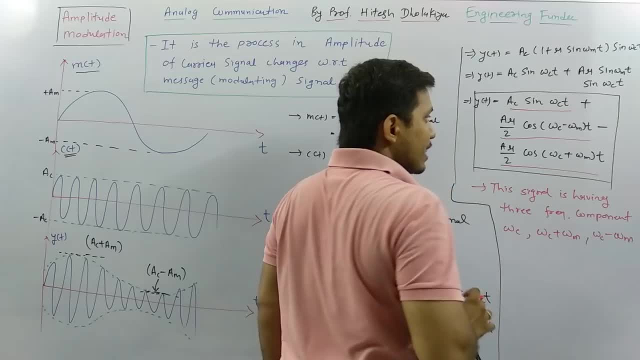 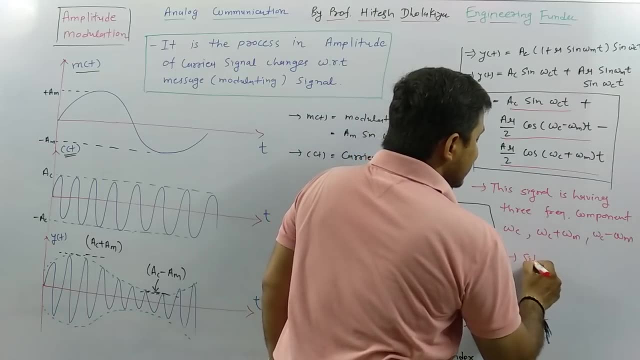 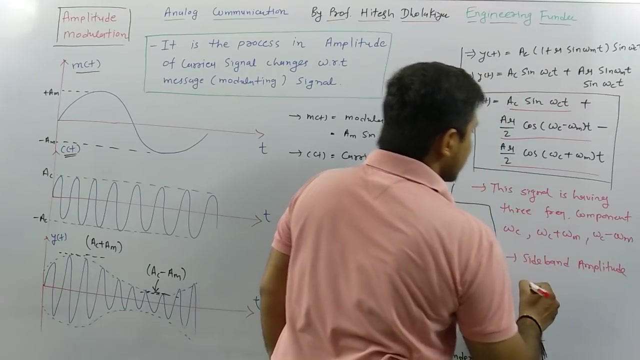 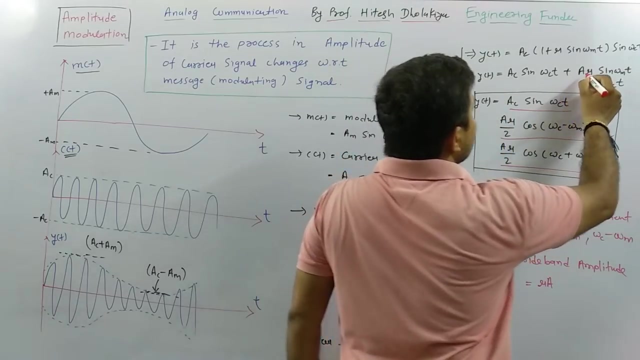 We can say omega C plus omega MT and omega C minus omega MT. These are sidebands, So sideband is having amplitude, Sideband amplitude, That is mu, A. This is what exactly AC and only A. It is AC, So mu, AC by 2.. 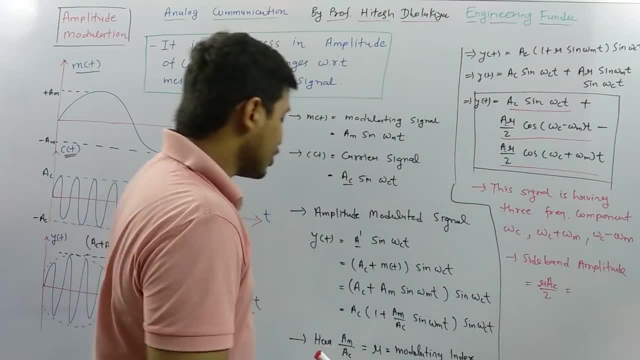 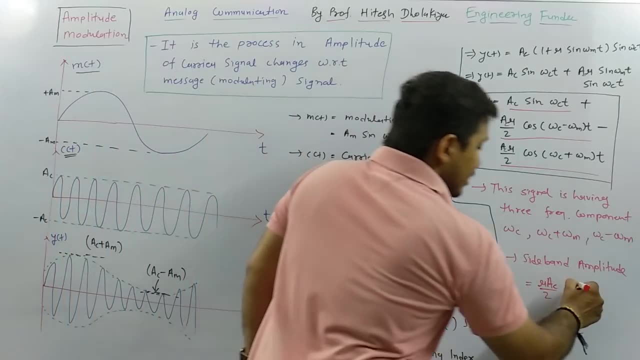 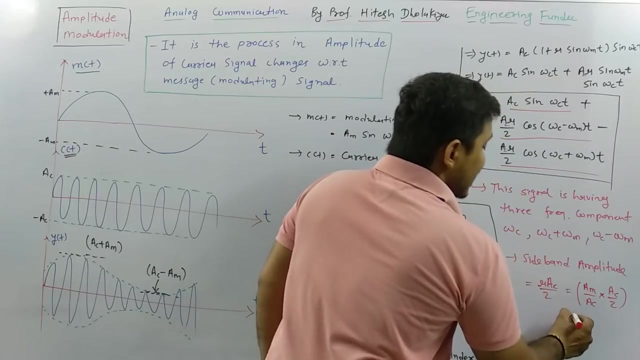 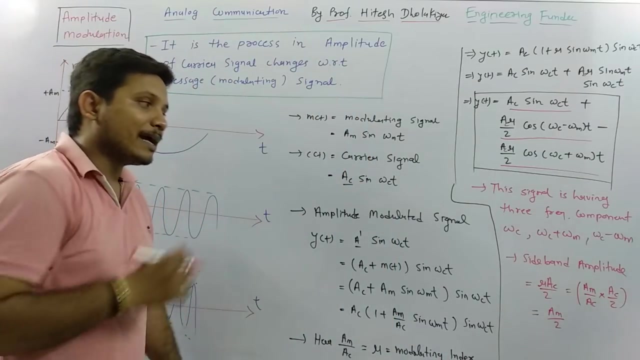 Mu is modulating index. That is modulating signal samplitude divided by carrier signal samplitude. So that will be AM by AC Into AC by 2.. So that is exactly AM by 2.. So this is what amplitude of sideband. 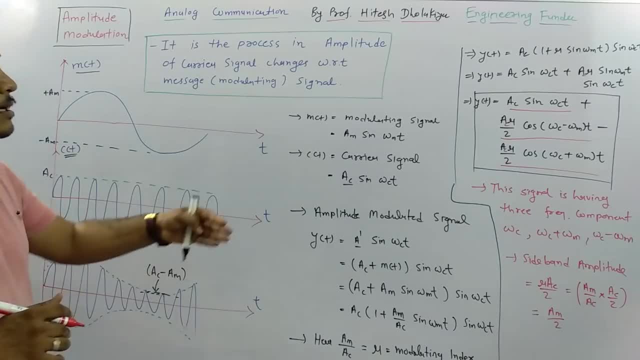 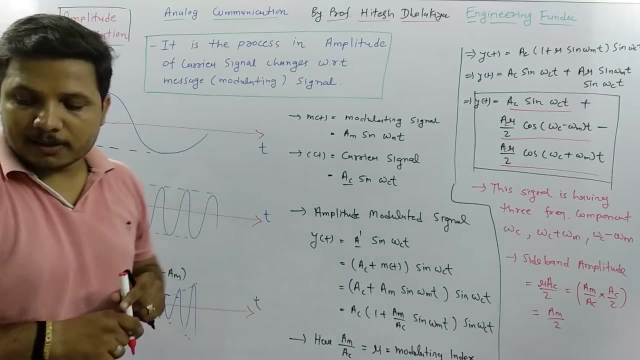 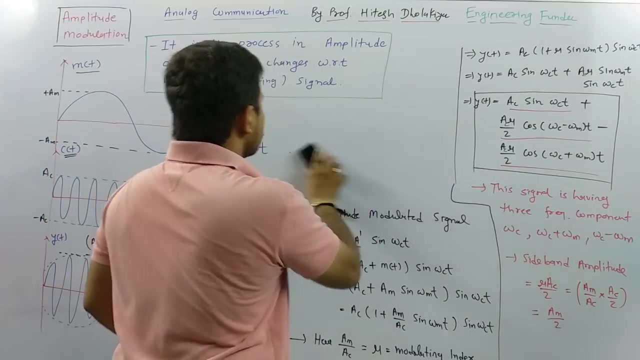 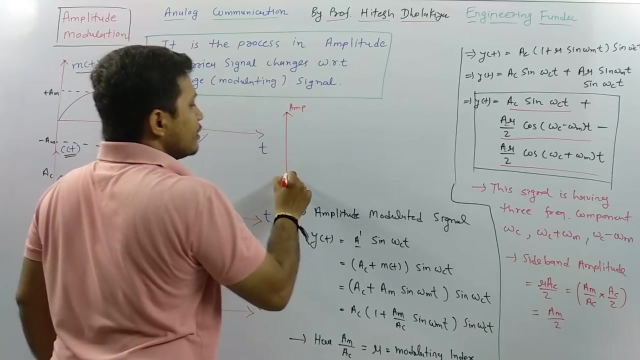 Now, as if we see this basic signal, which is what modulated signal, Then if you plot its frequency response, Then that frequency response that I am plotting it over here, So that will be, looks like: here that is amplitude and here that is frequency. 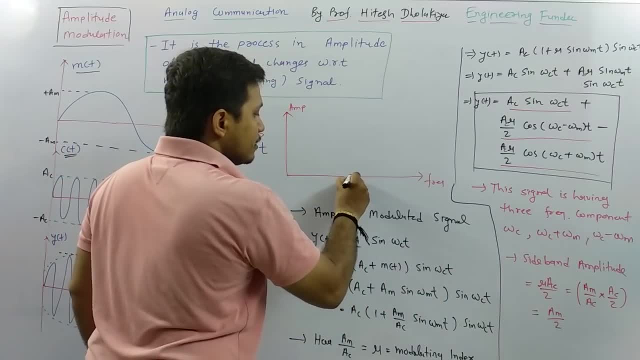 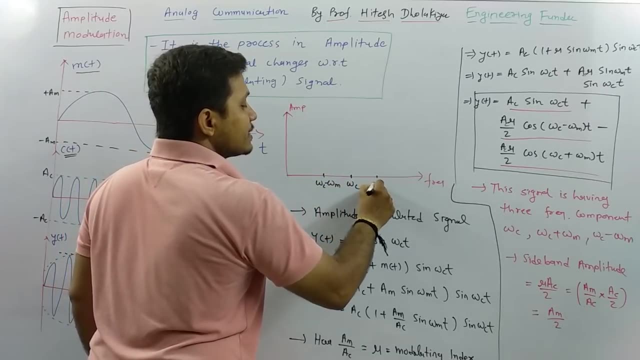 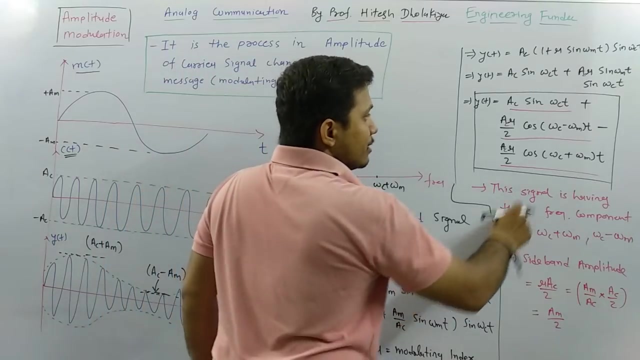 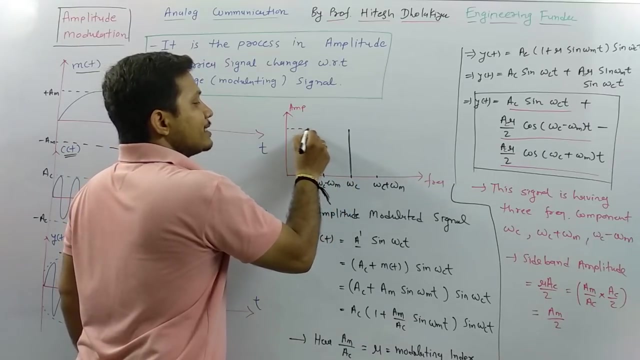 So there are three frequency component. This is omega C, This is omega C minus omega M, And here frequency component is omega C plus omega M. Omega C frequency component, That is having amplitude AC. So this is what amplitude which is there with carrier signal. 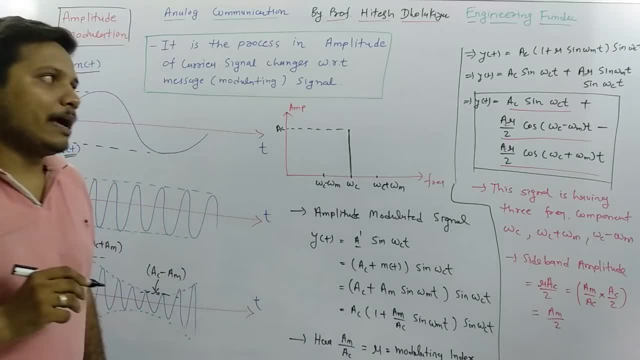 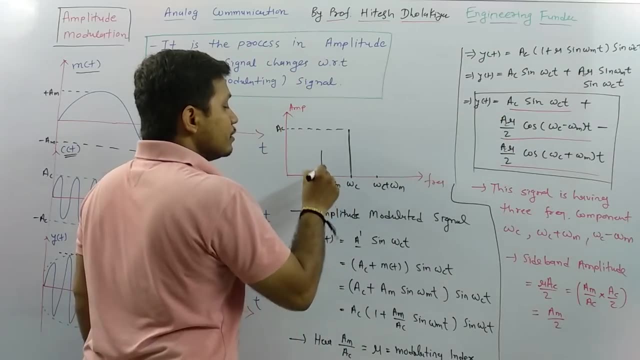 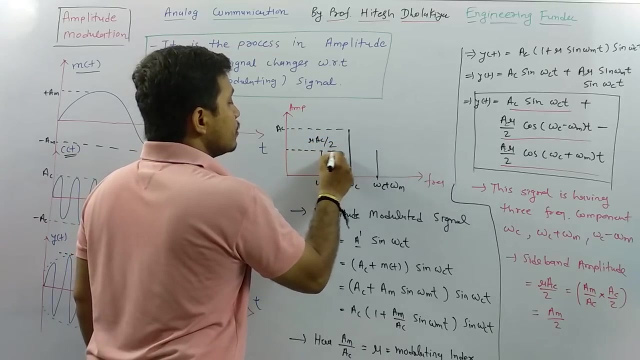 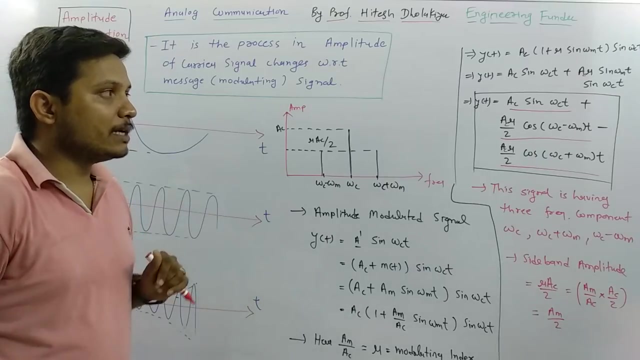 That is AC in amplitude, modulated signal And sidebands. that is having amplitude mu AC by 2.. Mu AC by 2.. So this is what amplitude which is there with sideband And that is omega C minus omega M and omega C plus omega M. 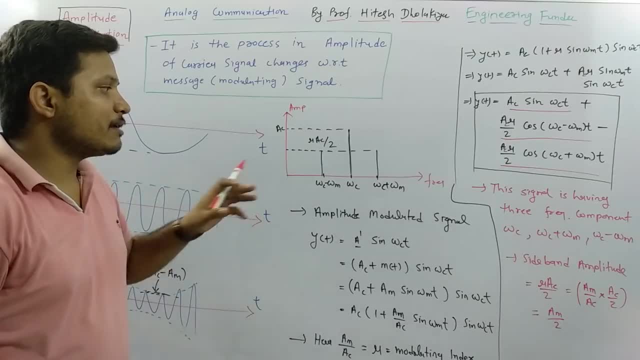 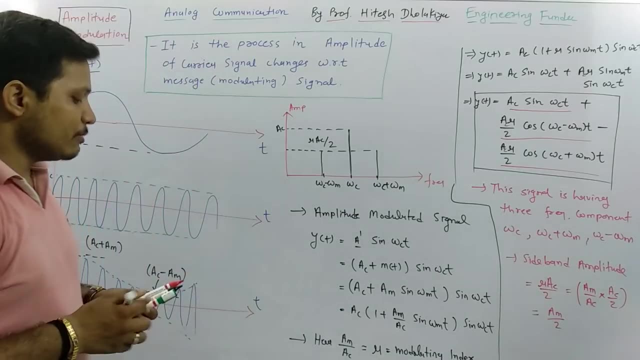 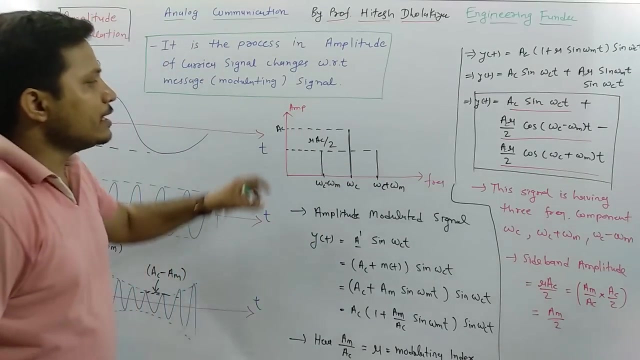 So that is what the amplitude which is there with sideband, Now here, few things that we need to discuss as a basics of amplitude modulated system. Now, in amplitude modulated signal, If you see, there are three things which we are sending. 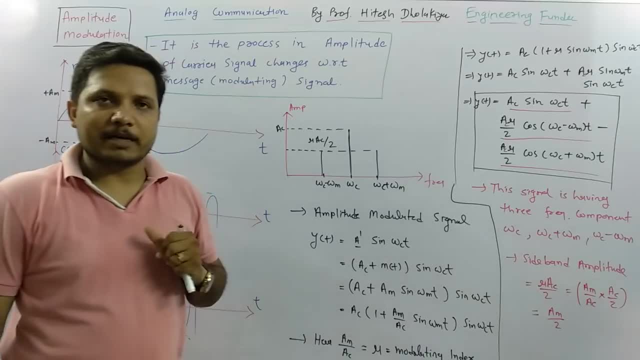 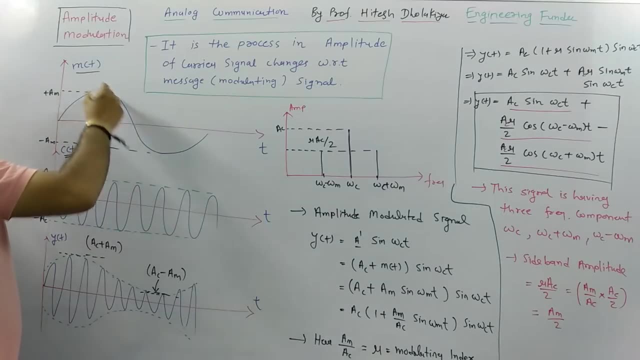 Carrier signal and sidebands. Now, carrier signal is not having information. You can see, information means message signal. So message signal that is having frequency, omega M, D. Carrier signal is AC sin, omega C, D. So the signal which we send by this component is not a information. 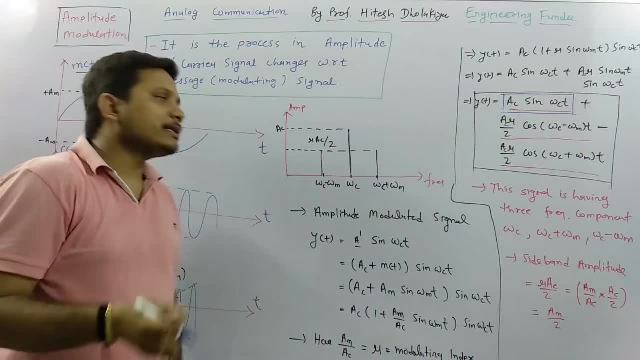 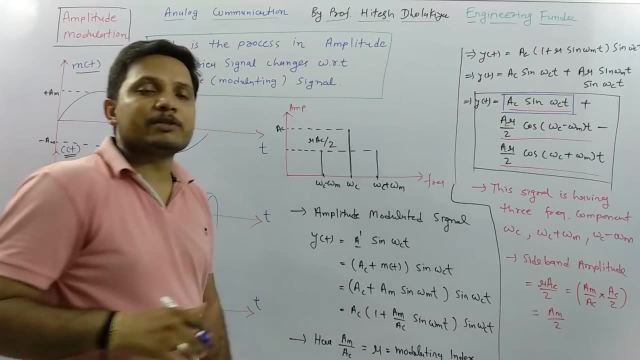 So this is not information. So when we send signal by amplitude modulated signal, In that case we send carrier signal. So that is what waste of power and major power that is there. with this You can see amplitude is more with omega C. 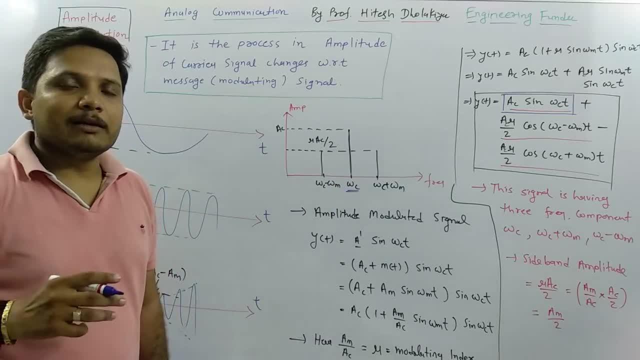 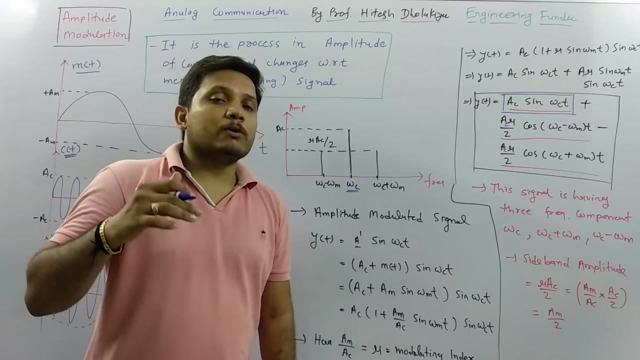 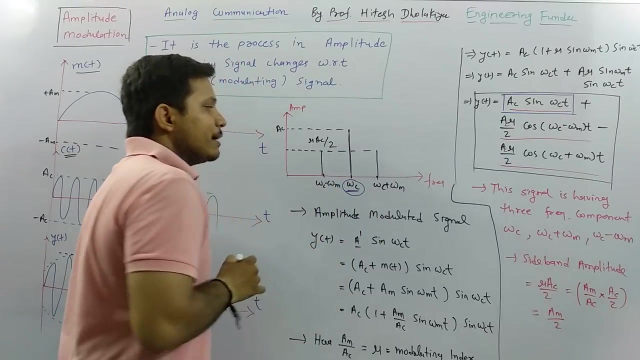 So amplitude modulated signal is having higher power. that is there with carrier signal And that is unwanted signal. So this is where some drawbacks are there with AM. So this is what the drawback which is there with AM, Which is sending AC. 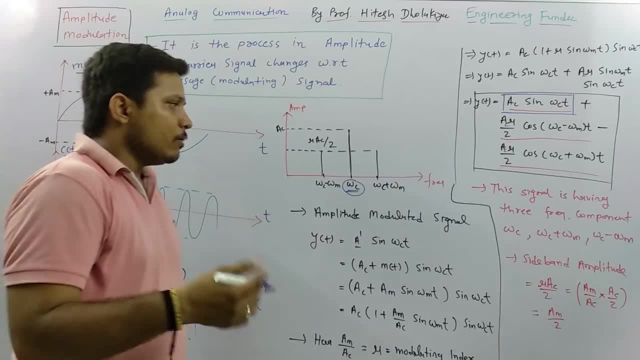 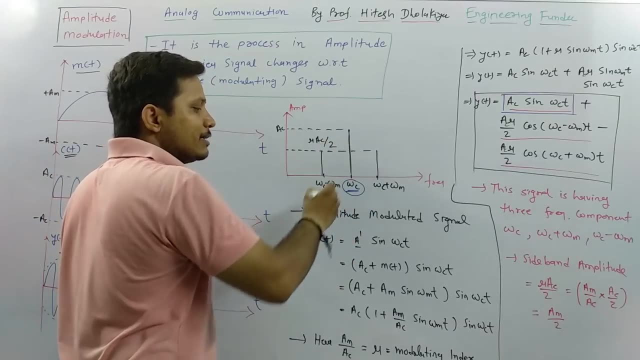 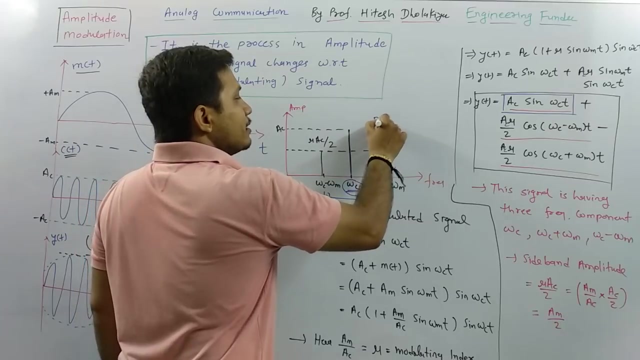 Sin: omega C, D, that is carrier signal. Now there are few more drawbacks, Like if you see the bandwidth of AM signal, Then this bandwidth is this much. Now, what is that bandwidth? That bandwidth is Bandwidth that is omega C minus omega M to omega C plus omega M. 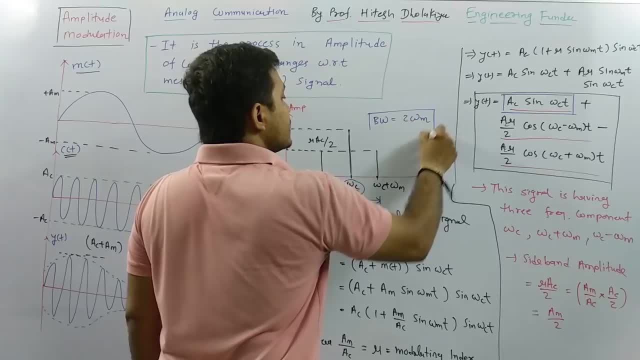 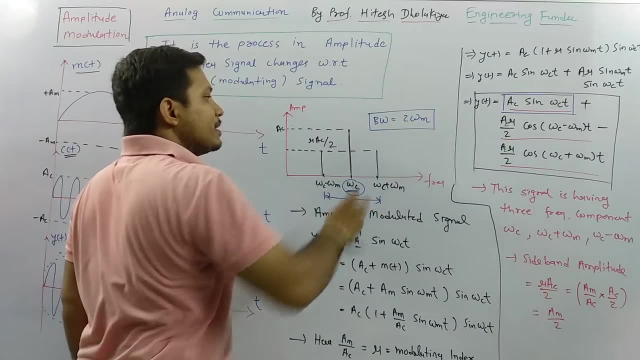 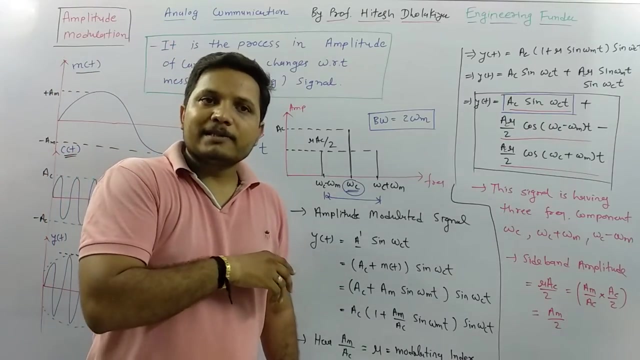 So it means it is 2 omega M. So this is what the bandwidth which is there With AM. So this bandwidth is higher bandwidth than the bandwidth of modulating signal. So when we talk about bandwidth of AM signal, 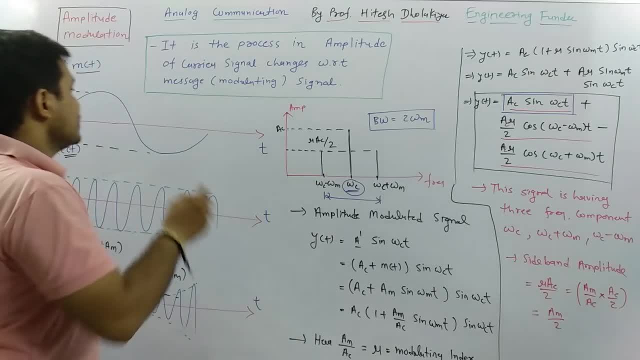 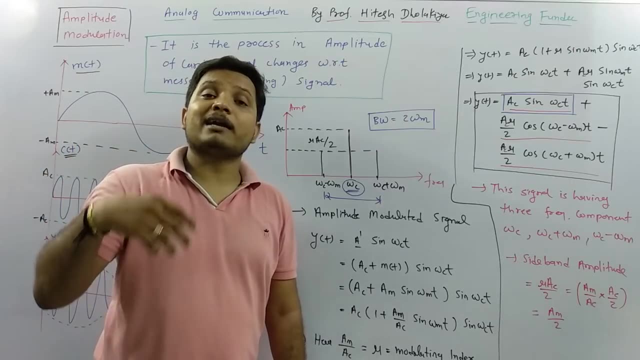 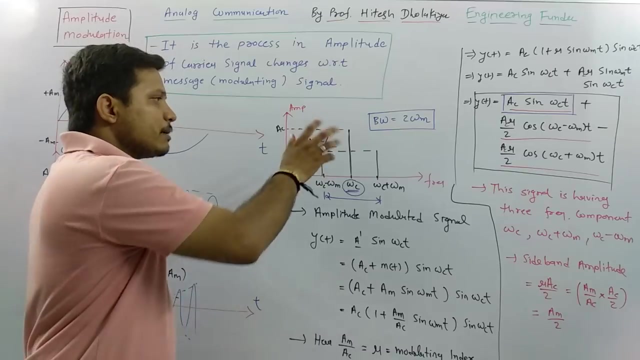 Then that bandwidth is double than the bandwidth which is there with signal, So it acquires higher bandwidth as well as this AM signal. That is, having higher amount of power which we need to transmit for wireless communication. So these are the basic problems which is there with AM. 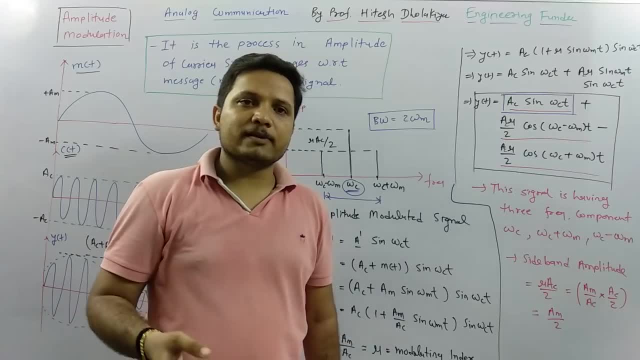 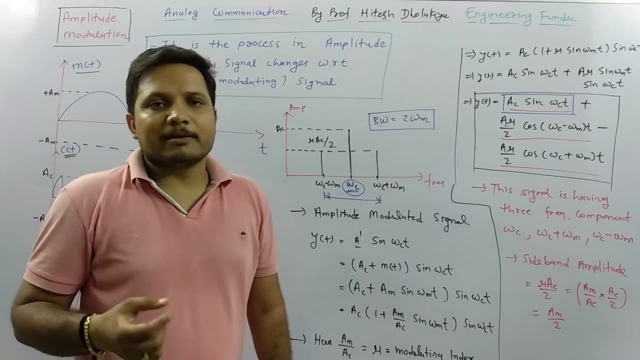 And to solve out those issues. There are few more techniques which is there with amplitude modulation. Those are double sideband suppress carrier as well as single sideband suppress carrier, So that I will explain in future videos. So in next sessions you will be finding 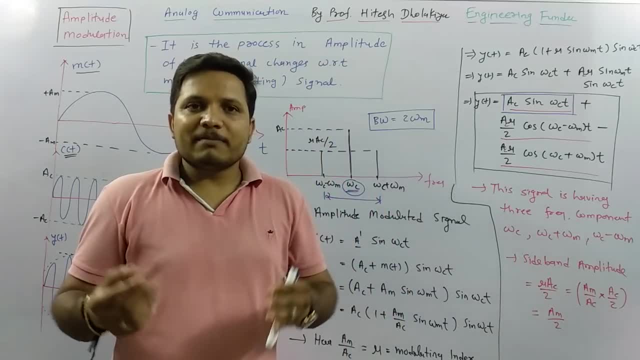 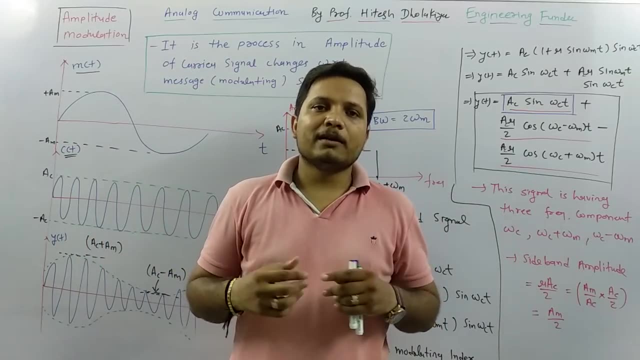 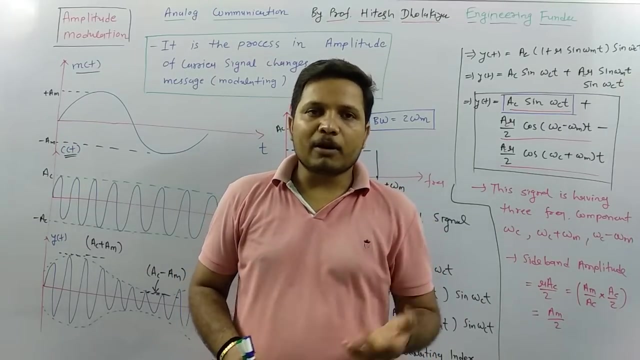 I will be explaining you: DSBSC double sideband suppress carrier And SSBSC single sideband suppress. So that is what I will be explaining in next few sessions, So stay tuned with this. So one should have basic idea about what is AM- amplitude modulation. 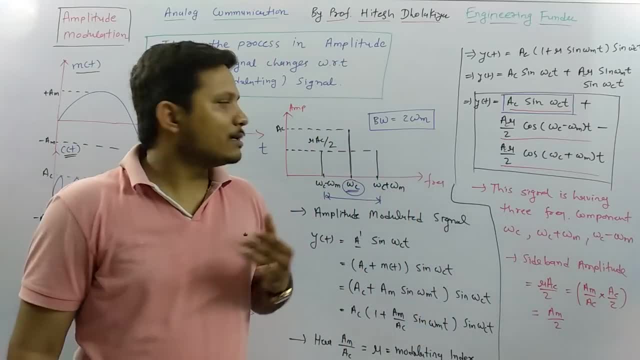 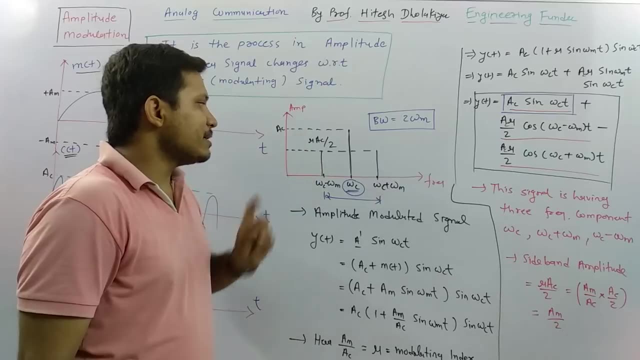 And that is what sending carrier signal plus sideband signals. So this is what sideband signal- omega C plus omega M and omega C minus omega M, And its amplitude is mu AC by 2.. Now here, few more things that we need to focus about. 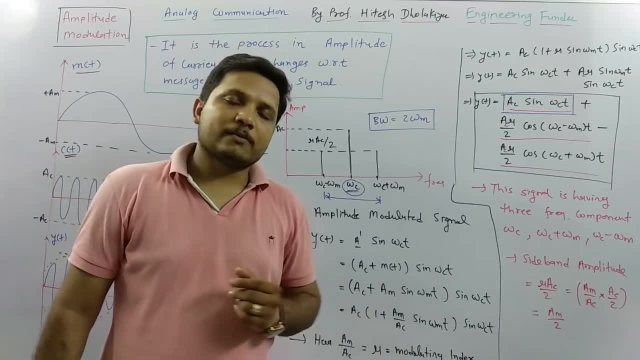 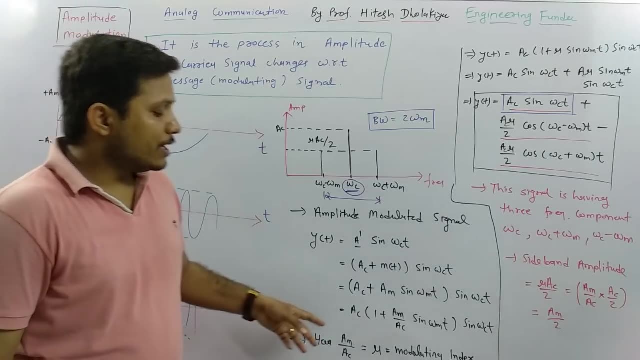 One is modulating index. Now, what is modulating index? Amplitude of modulating signal divided by amplitude of carrier signal. So here, modulating index that should be lower than 1.. Modulating index that should be lower than 1.. 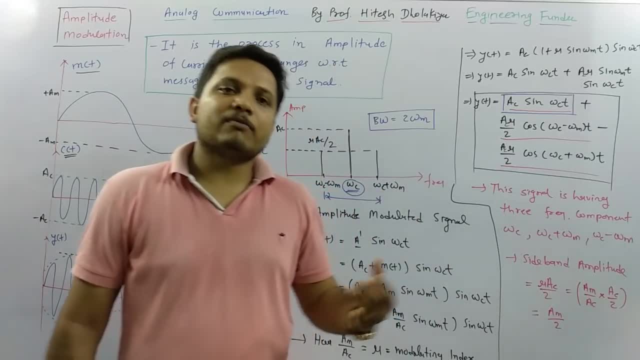 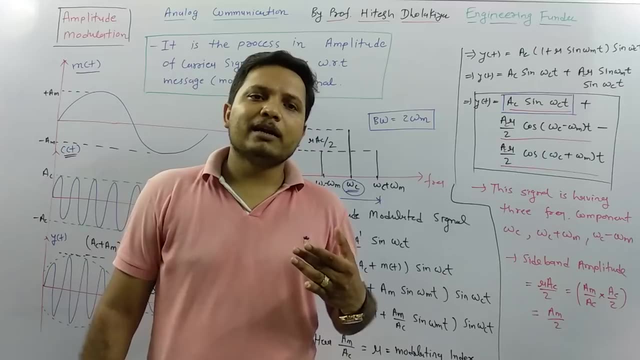 Otherwise there will be phase distortion. that will be there with amplitude modulated signal, So that we will be discussing in few of next sessions Where you will come to know, like why there should be modulating index which should be lower than unity.